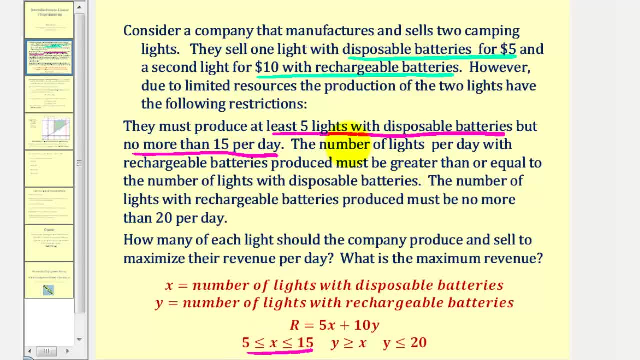 less than or equal to fifteen. Next, the number of lights per day with rechargeable batteries produced must be greater than or equal to the number of lights with disposable batteries, And therefore y must be greater than or equal to x. Remember, y is the number of lights with rechargeable batteries. 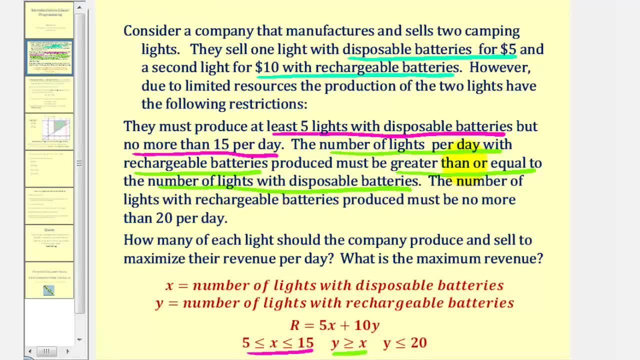 And then, finally, the number of lights with rechargeable batteries must be no more than twenty per day, which means y must be less than or equal to twenty. So this is all the given information from our problem. So linear programming or linear optimization. 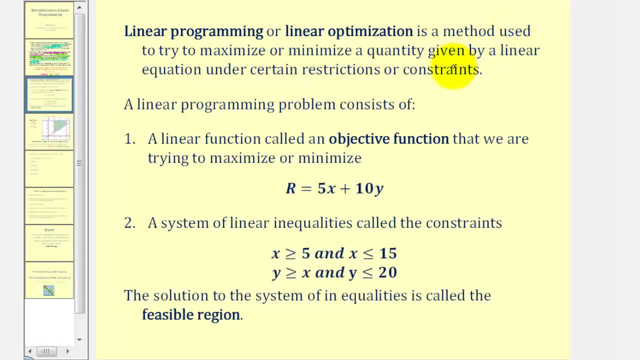 is a method used to try to maximize or minimize a quantity given by a linear equation under certain restrictions or constraints, which is what we have here. That's what we had in the previous problem. A linear programming problem always consists of number one. 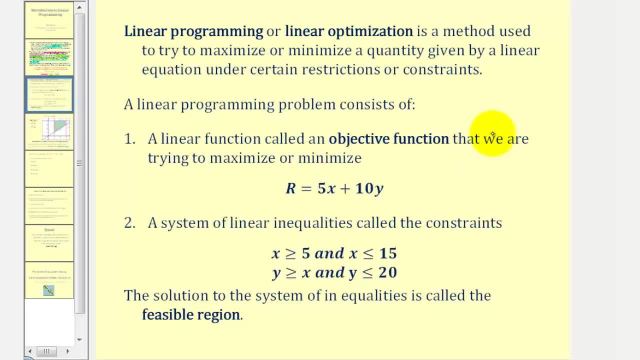 a linear function, called an objective function, that we are trying to maximize or minimize. So in our previous example, r equals five x plus ten. y is our objective function, which we're trying to maximize. A linear programming problem also has a system of linear inequalities called the constraints. 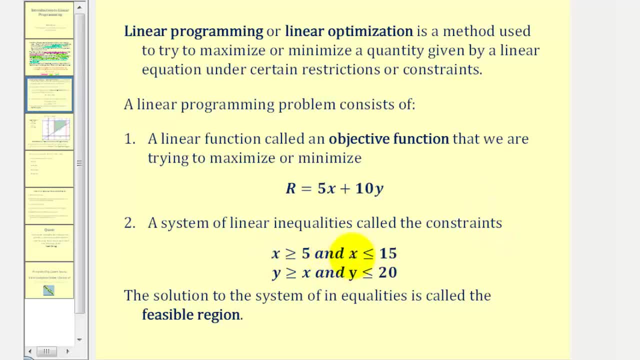 In our case we had x is greater than or equal to five and less than or equal to fifteen, as well as y must be greater than or equal to x and y must be less than or equal to twenty. So these are the constraints. 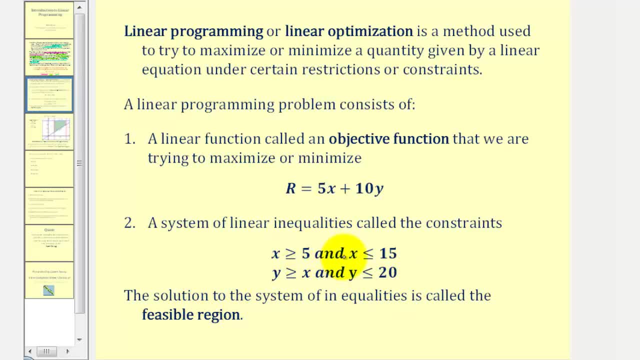 And the solution to this system of inequalities here is called the feasible region. So for the next step, we'll graph the feasible region by determining the solution to the system of inequalities, And to save some time, I've already graphed this, which we see here. 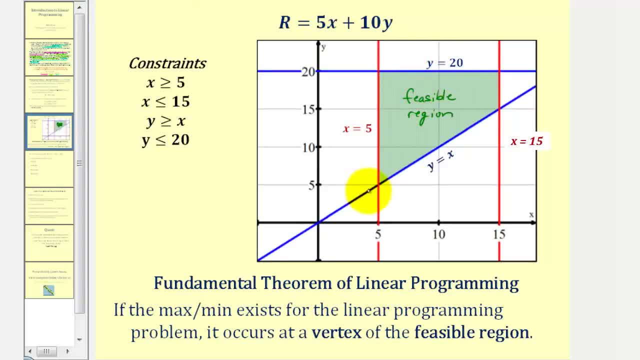 This green region. here is the feasible region. Let's review how this is found, Because we have four inequalities here. we would graph all four inequalities and look for the region that is shaded four times. So for this first inequality, x is greater than or equal to five. 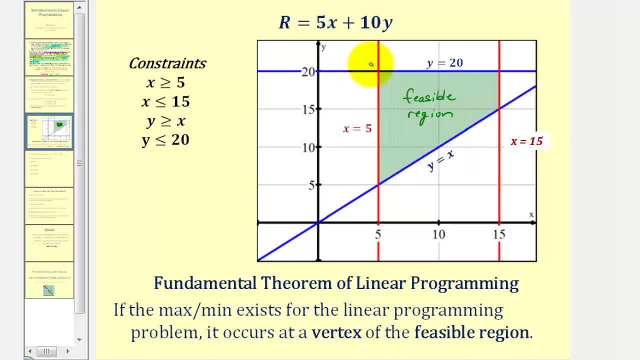 because of the equal part, we'd have a solid vertical line here at x equals five, And because this x is greater than or equal to five, we would shade to the right of this vertical red line. Next we have x. also has to be less than or equal to fifteen. 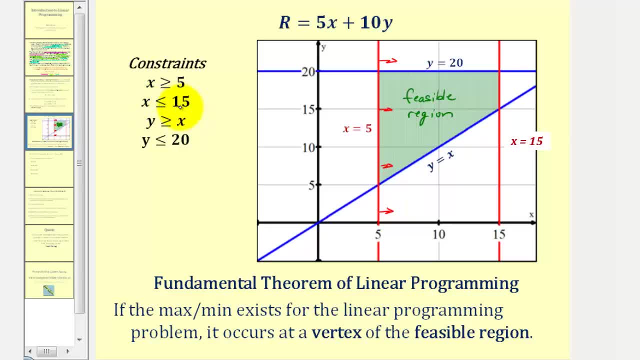 So we'd graph the vertical line x equals fifteen, which is this red vertical line, And because we have x is less than or equal to fifteen, we would shade to the left or in this direction here. Next, we have y is greater than or equal to x. 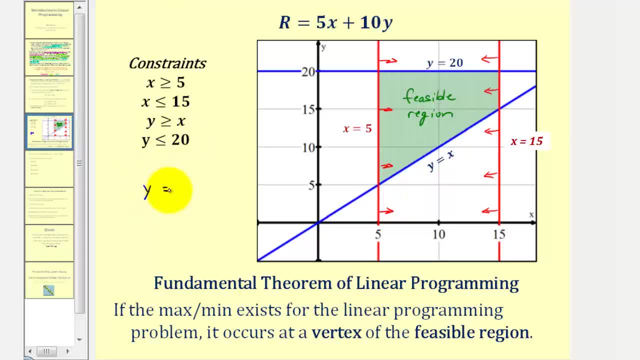 If we begin by graphing the line y equals x, which, if we want, we can write as y equals one, x plus zero, which tells us the y intercept is zero and the slope is one. So this would be the line y equals x. 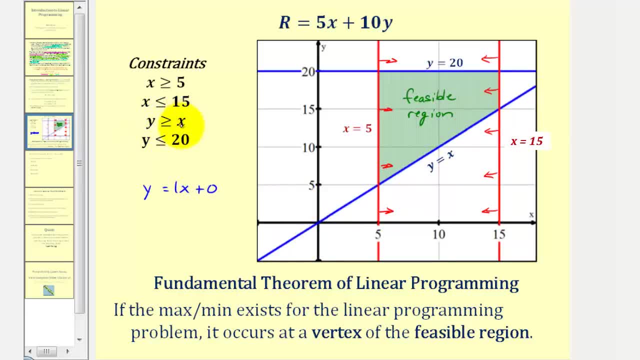 But because the inequality is y is greater than or equal to x, we would shade above the blue line or this half plane here, And then finally we have y is less than or equal to twenty. Well, y equals twenty would be this horizontal blue line. 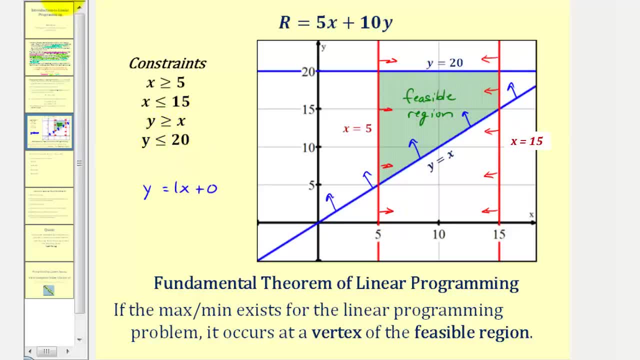 And because of this, because we have y is less than or equal to twenty, we would shade below this horizontal line. So the region that's shaded four times or the region that satisfies all these inequalities at the same time once again, is this region here? 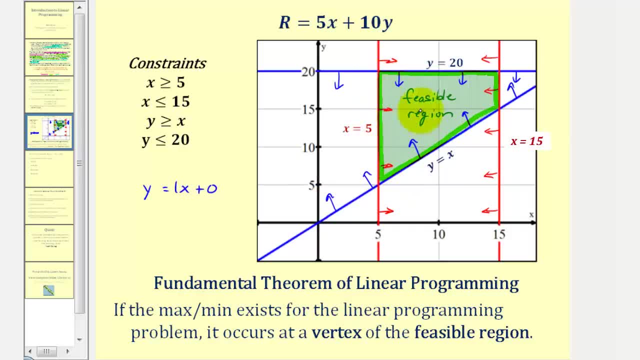 Called the feasible region. Now, the most important idea about linear programming is the fundamental theorem of linear programming, which states: if the maximum or minimum exists for the linear programming problem, it occurs at a vertex of the feasible region, Which in our case means: 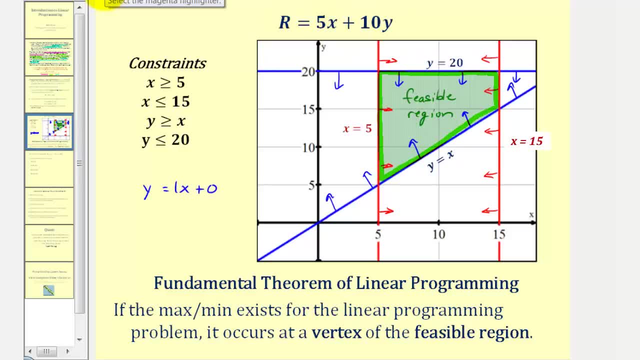 the value of x and y that will maximize our revenue would have to be one of the corners or vertices of our feasible region, Which would be this point, this point, this point or this point. So now we find the coordinates of these four points. 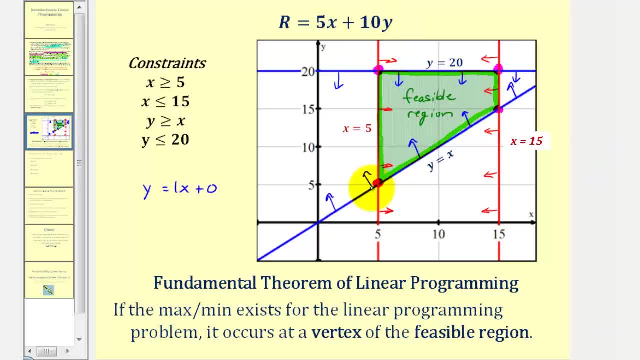 sub those x and y values into our revenue equation and whatever coordinates give us, the largest revenue would be the value of x and y. that would maximize the revenue from the given constraints. Now, many times we do have to solve a system of equations. 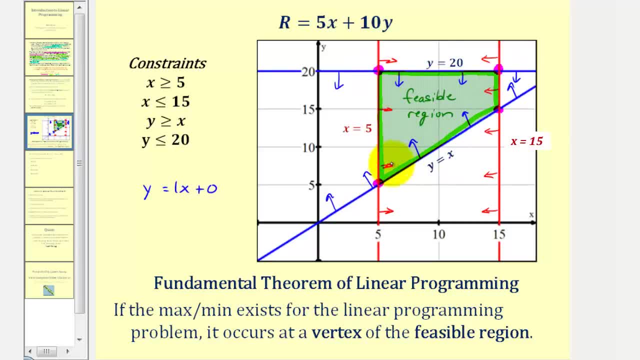 in order to find the coordinates of these vertices. but notice, in this case we can easily determine the coordinates from the graph. Notice how this point would have coordinates five comma five. this point would have coordinates fifteen comma fifteen. this point would have coordinates fifteen comma twenty. 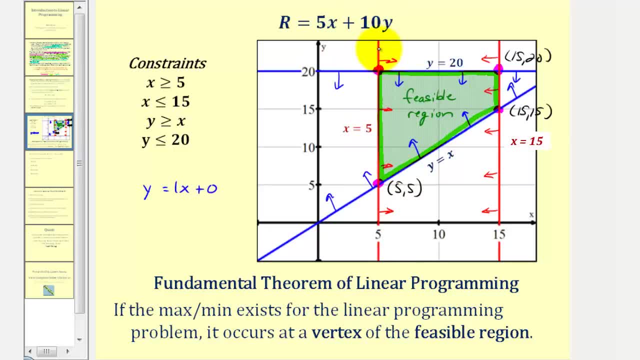 and this point would have coordinates five comma twenty. In our next several examples, though, we will have to, we will have to. in the next few examples, though, we will have to use algebra in order to find the coordinates of these vertices. 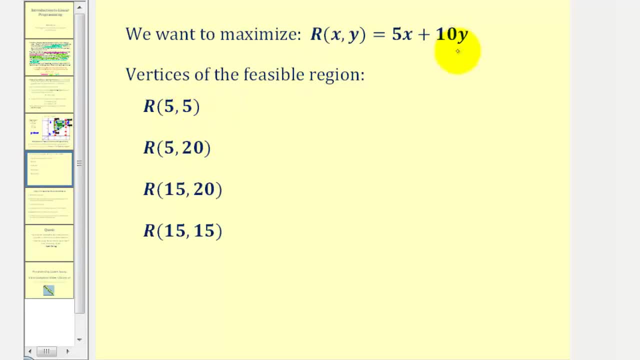 So now we'll substitute the x and y values into our revenue equation to determine how many of each flashlights the company should produce and sell to maximize the revenue When we have a function in terms of two variables, sometimes we'll see it written in this form here: 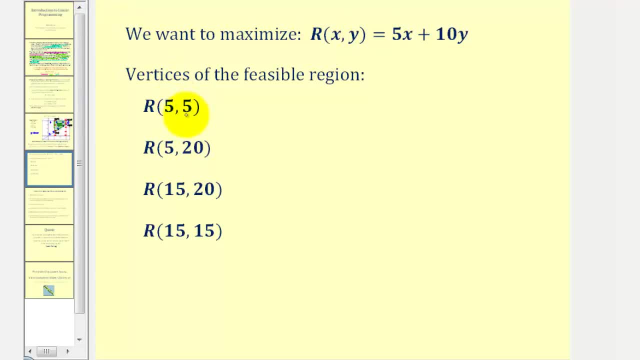 So for r of five comma five, we'll substitute five for x and five for y, which would give us five times five plus ten times five, and this would be twenty five plus fifty or seventy five. So this tells us that if the company 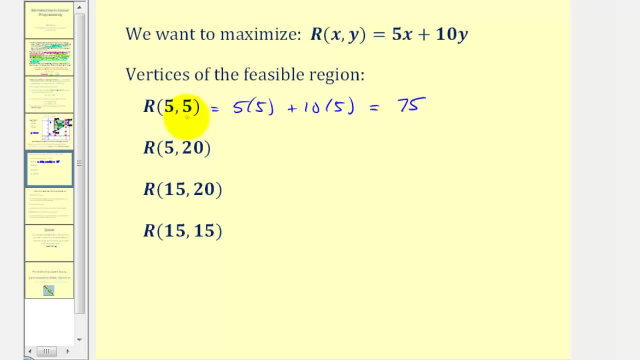 produces and sells five of each flashlight, the revenue would be seventy five dollars per day. For r of five comma twenty, we would have five times five plus ten times twenty. well, five times five is twenty five, ten times twenty is two hundred. 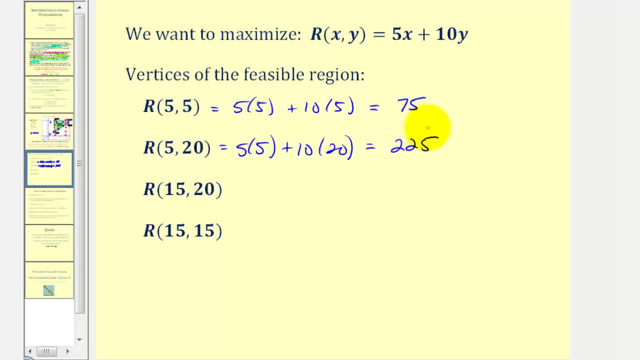 so we have two hundred twenty five. Next we have r of fifteen comma twenty, so we'd have five times fifteen plus ten times twenty, so this would be seventy five plus two hundred or two hundred seventy five. Then finally, r of fifteen comma fifteen. 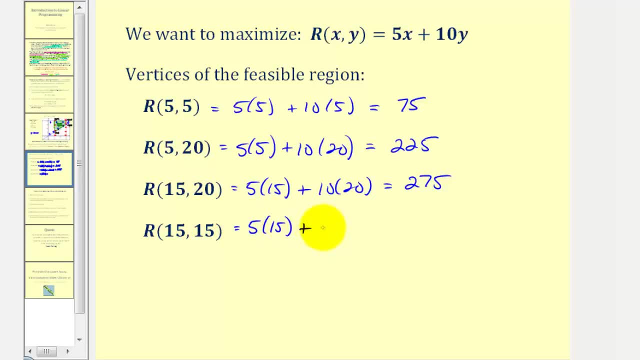 we'd have five times fifteen plus ten times fifteen, which would be seventy five plus one hundred fifty or two hundred twenty five. So notice how we have the largest revenue per day here, at two hundred seventy five dollars per day. let's go ahead and label the units here. 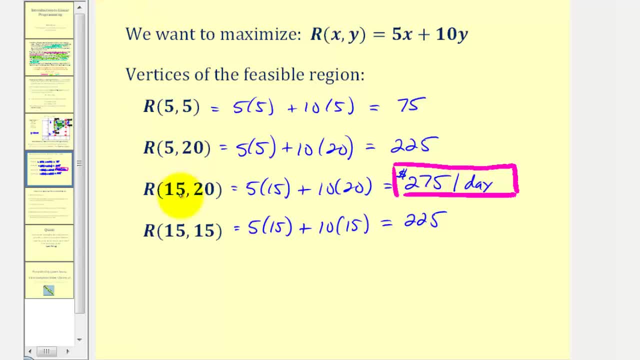 And this maximum revenue occurs when the company produces and sells fifteen lights with disposable batteries and twenty lights with rechargeable batteries. So let's go ahead and summarize this To maximize revenue at two hundred seventy five dollars per day. the company